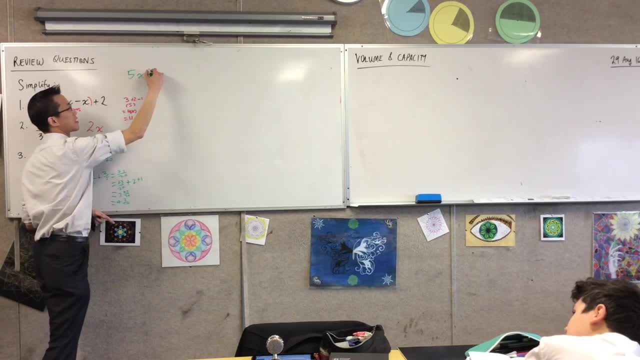 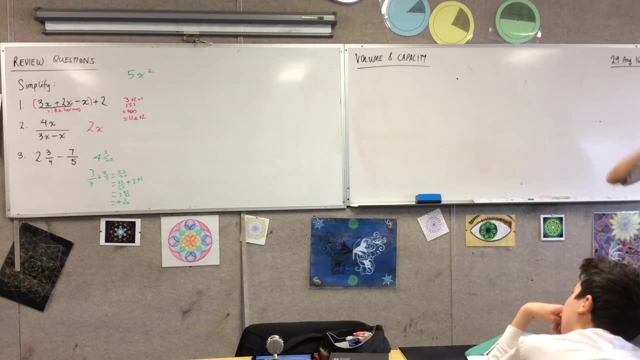 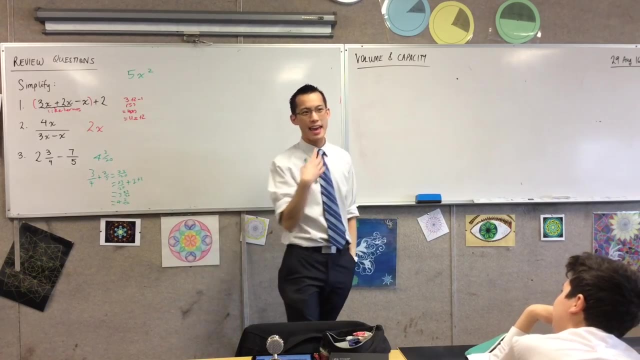 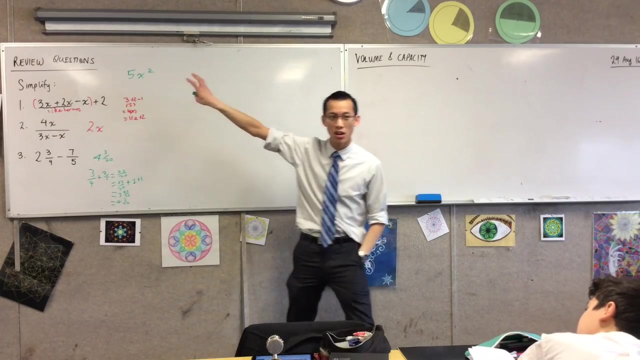 And then x and x. I know what happens when it's x and x, It's x squared. Now my question to you is: why? is because Jaron's way of approaching it is exactly right? why is Jaron's approach right and why is this one not valid? Can anyone give me an explanation, Not just a rule, but an explanation- as to why it's not this? What do you reckon, Rish? 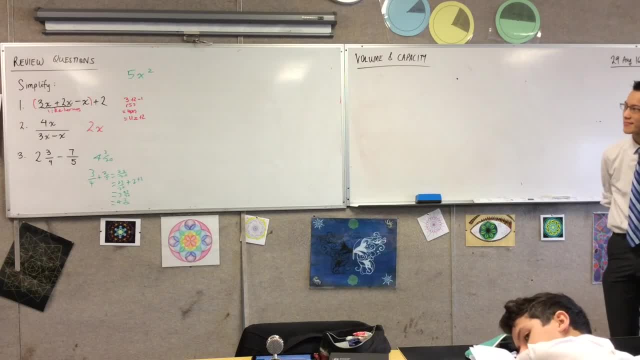 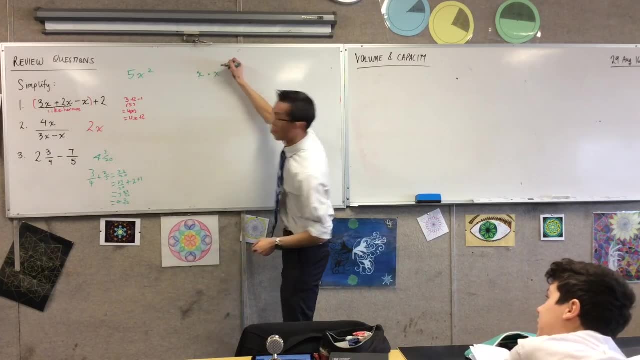 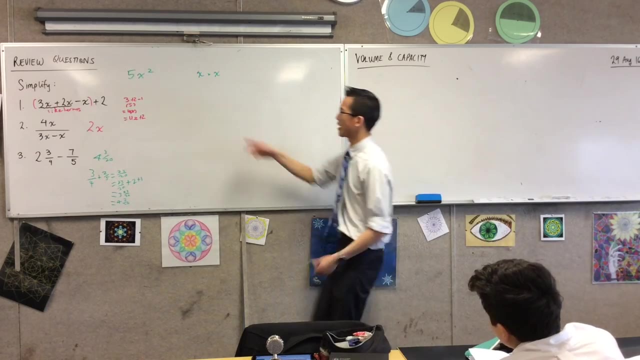 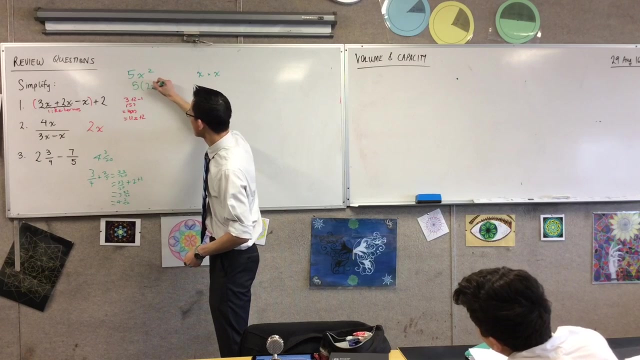 Because x squared, What is x times 2?? I mean, yeah, x times x. Okay, alright, But hold on a second. Hold on a second. Why shouldn't I multiply them together? Why, you know, like, if you want me to add them instead, then shouldn't it be 5 and 2x? Isn't that what it should be? Why isn't it that? What do you reckon, Frank? 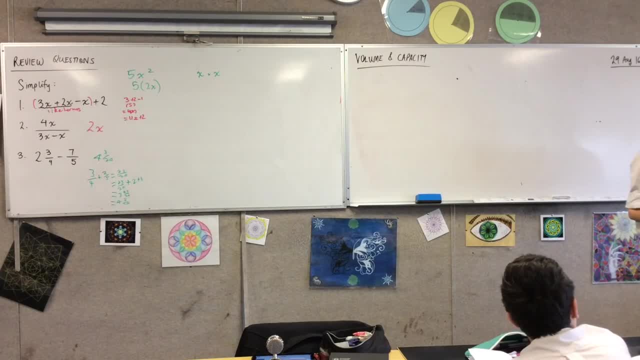 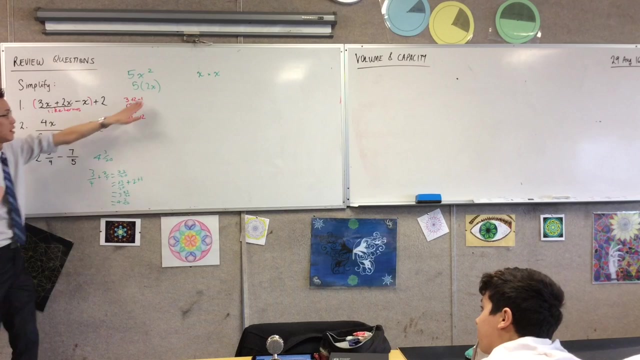 Um, well, you know, the tattoo has to be 5.. No, no, not yet, Especially because we're not focused on this right now. By the logic that I've just heard, right, 3 plus 2 is 5.. x plus x, if you want me to do addition, not multiplication, is 2x. So why isn't it this? Someone explain why it's not? What do you reckon, Jaron? 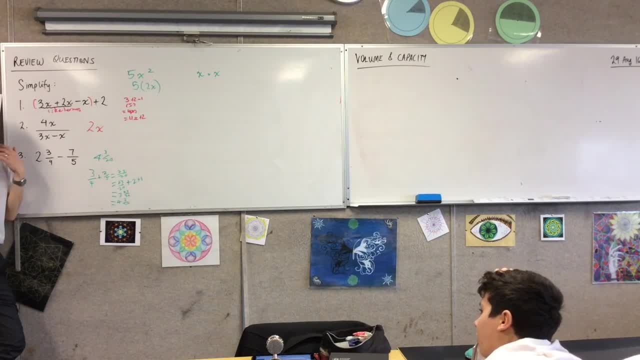 Because we don't know the number. So you mean it's about to do with like it's a variable, It's a pronoun, I don't know what's there. Hmm, So does that mean sometimes I can do that and sometimes I can't? 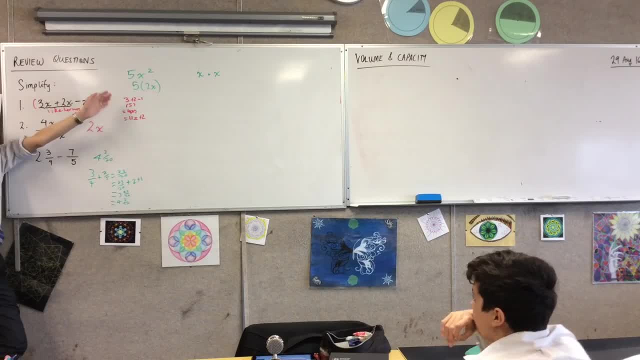 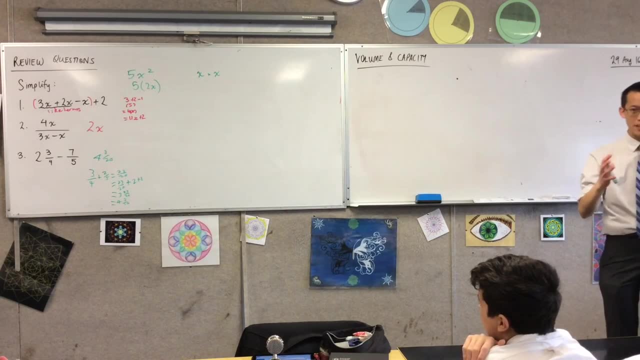 Is it a number? Could I do that? No, But why not? You've told me it's not multiplication. Okay, I'm alright with that, But if you add the 3 and the 2, why don't you add the x's? This is a really important question. Yeah, what do you want? 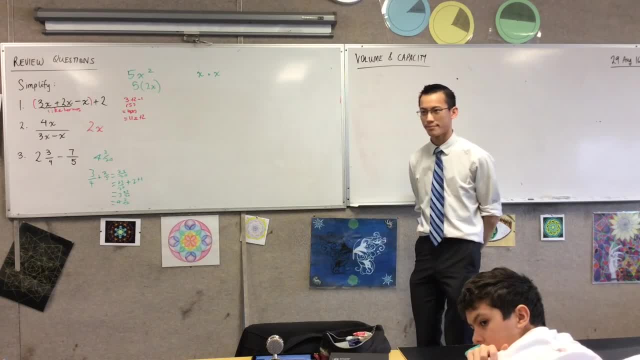 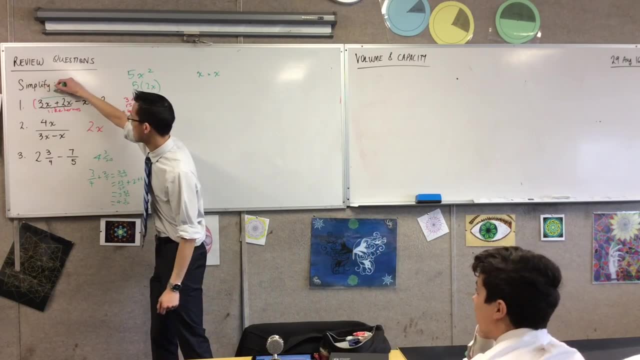 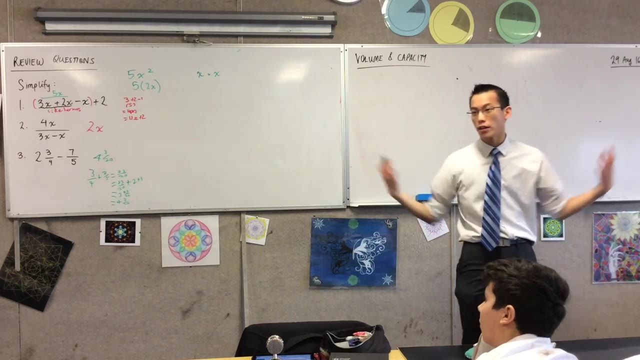 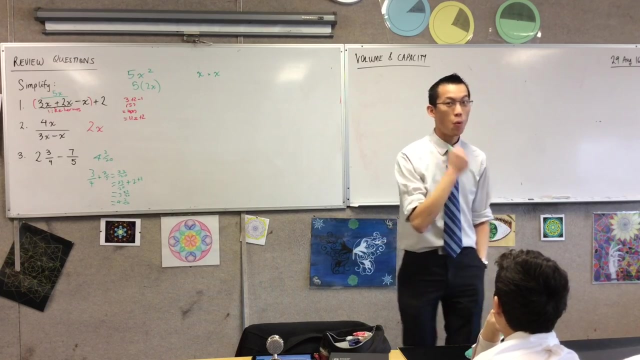 Because the x like symbolises 5 times x. So, um, So you're talking about just these guys being 5 times x. Okay, now can I? I might get one more try from Maria. It's interesting. There are lots of right things, but so far no one's actually explained to me why I shouldn't add these ones and then add those ones. So far, no explanation. What do you reckon? 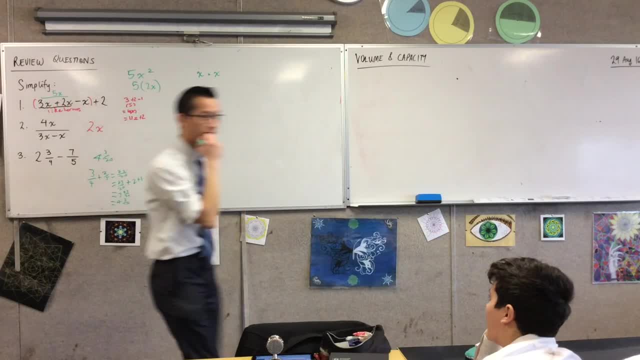 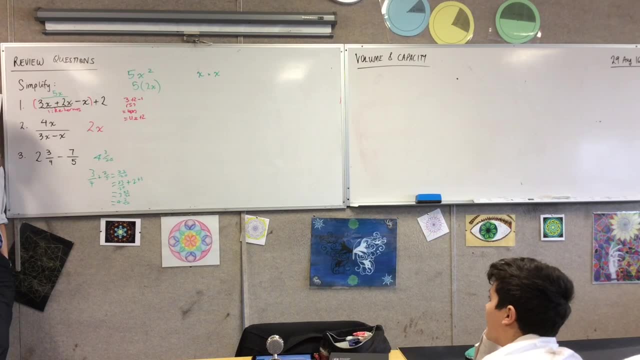 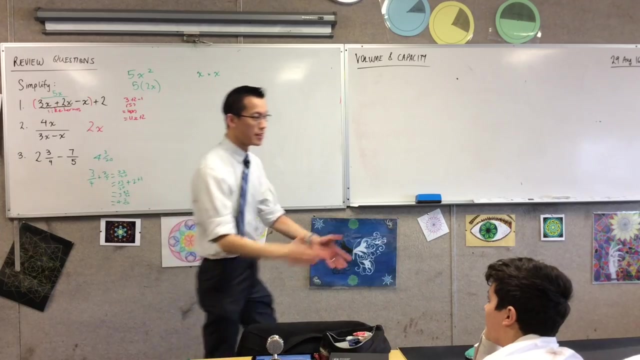 Is it because x equals something times that? Hmm, Now can I just suggest? By the way, I did ask for all laptops to be down and pens out of hands. Thank you, This is a really important moment. This year, we have learnt algebra. Algebra is a superpower. It's a superpower that lets you deal with all numbers when you don't even know what they are. 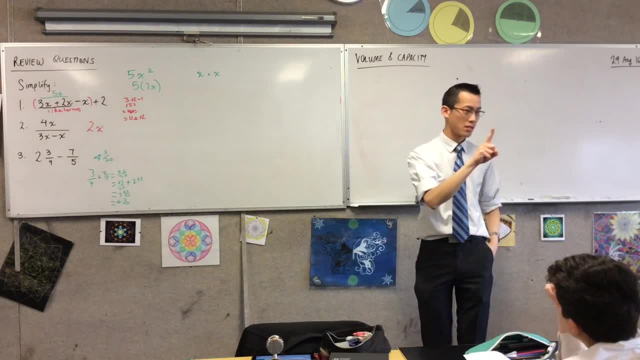 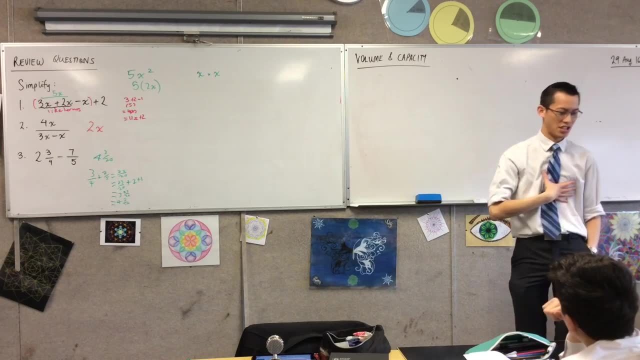 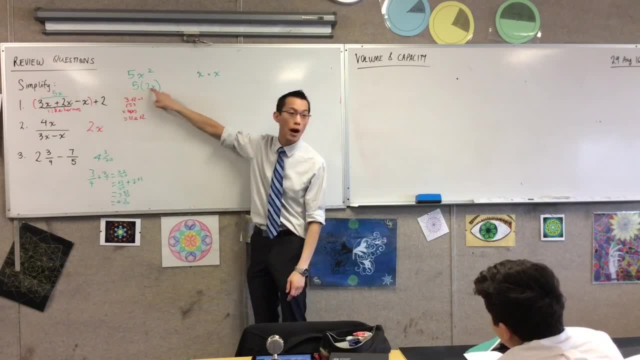 Why, Why, Why, Why, Why. No one has really given me a successful argument as to why it's not this. You added the 3 and the 2, that's how you got 5.. Do you agree with that? 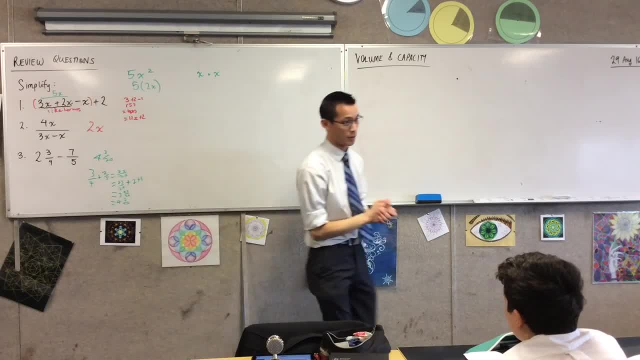 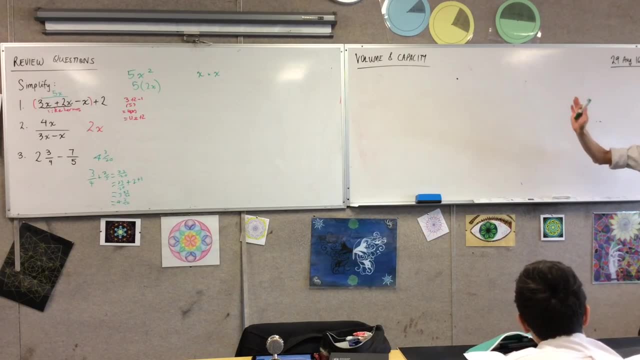 So why don't you add the x's? Okay, I will give you my explanation as to why. I'll write it to you, Maybe where you've got your working out, and you should definitely have written the question. by the way, If you haven't written the question, write it now, so I'll let you. 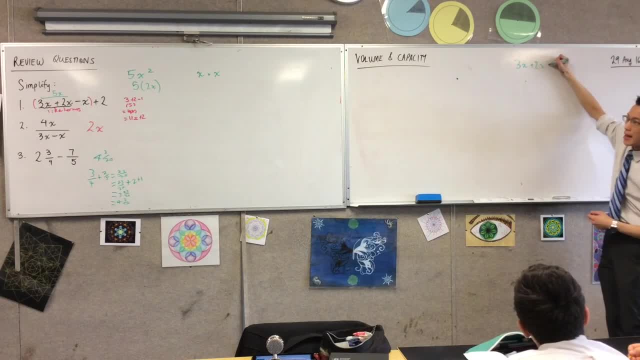 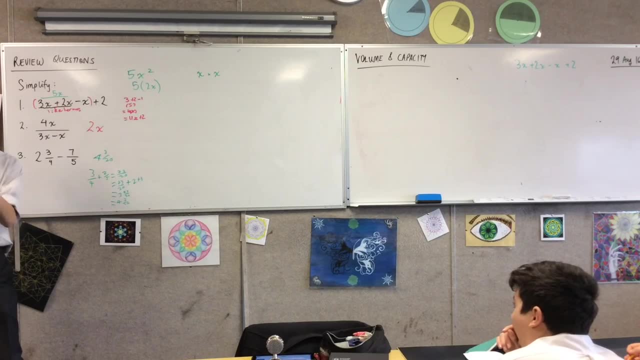 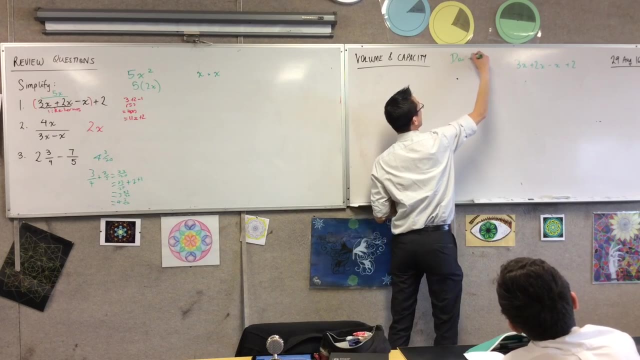 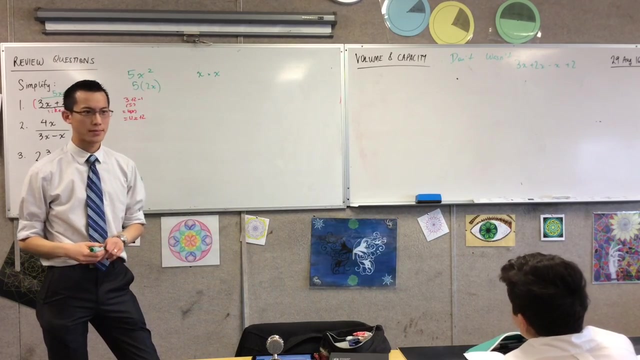 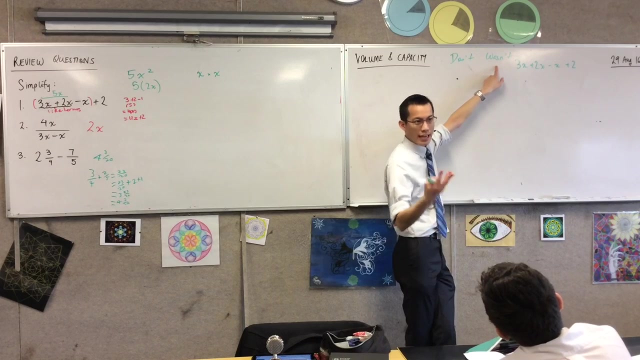 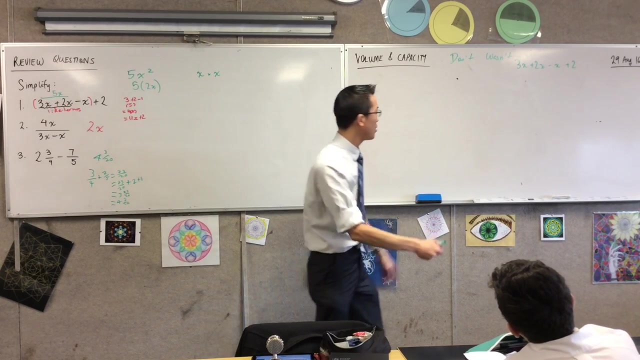 pick up your pens again. Here's my explanation as to why those first two terms do become 5x and not 5. lots of 2x. Let me ask you this question: 3x, It's shorthand. It's shorthand the way. don't or wasn't are shorthand. They're an abbreviation What's don't? an abbreviation of Do not, Very good. So I've omitted the o right. What about this? one Wasn't Okay, so again it's an o right Now. 3x. something has been omitted. What's been omitted? Christian Multiplication. 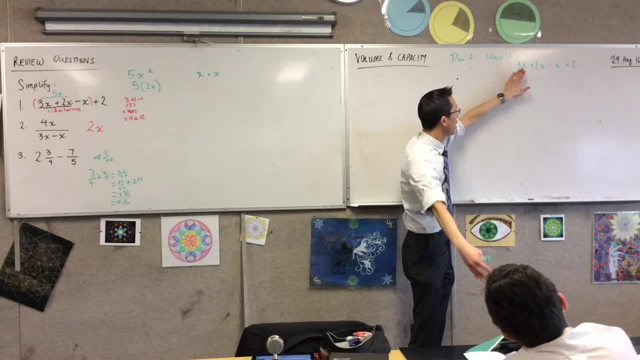 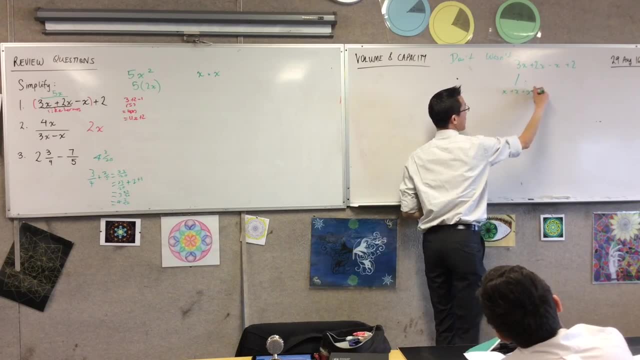 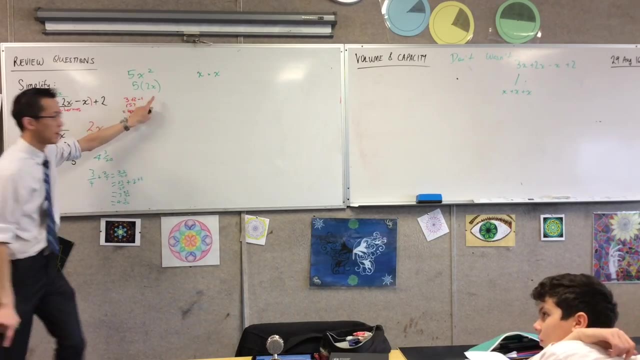 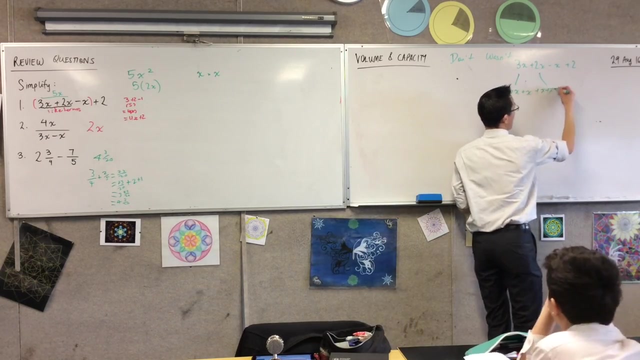 Multiplication. This is 3 times x, 3- lots of x, right? Which means I should be able to rewrite 3x as x plus x plus x. Do you agree? Yes, Right, Aha, Okay, Are the gears turning now? Now do you see why you can explain. it's not this. If 3x, is that what's 2x? It's x plus x, right? There are five things there. What are they? Five x's, Not five 2x's. 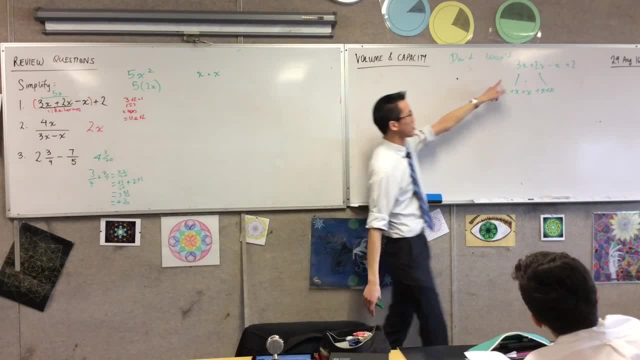 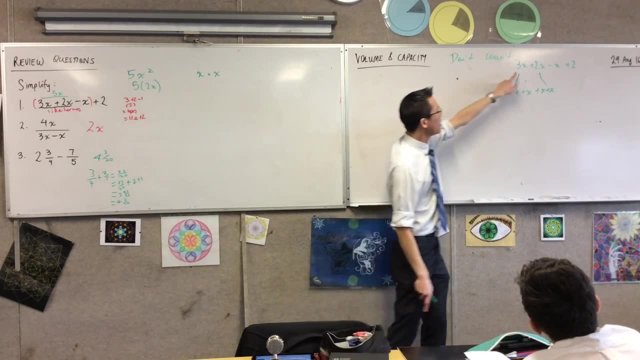 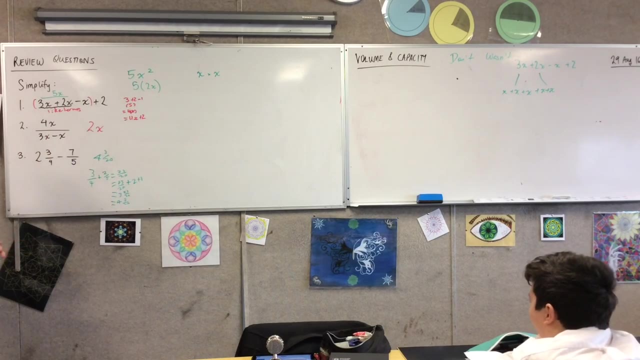 Right. So this is really important. It's not just a rule that someone told you you add these, but not these, right? What you need to think of is: what is it actually right? What is this shorthand for? Because it's a powerful language, so long as you actually understand it. Okay, I'm a bit more satisfied now. 5x, your takeaway. what x? Just 1x, right? 1x. Again, this is shorthand. There's a 1 and there's a multiplication sign. 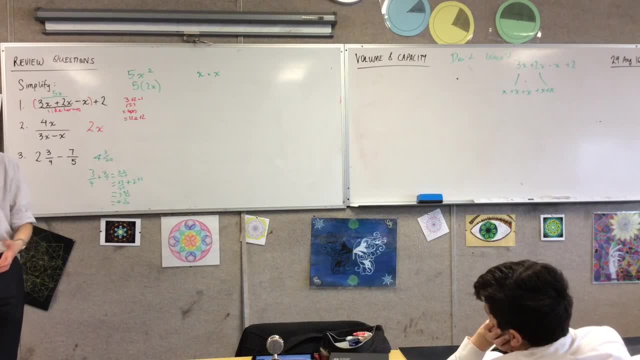 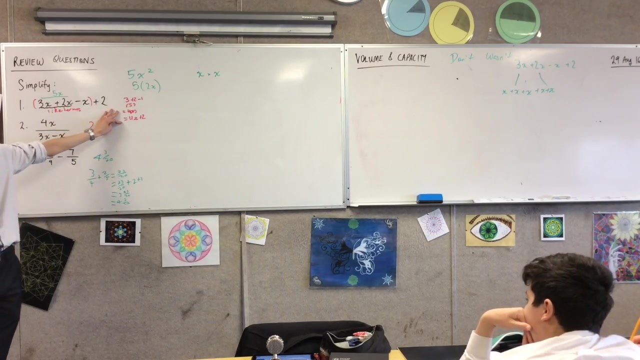 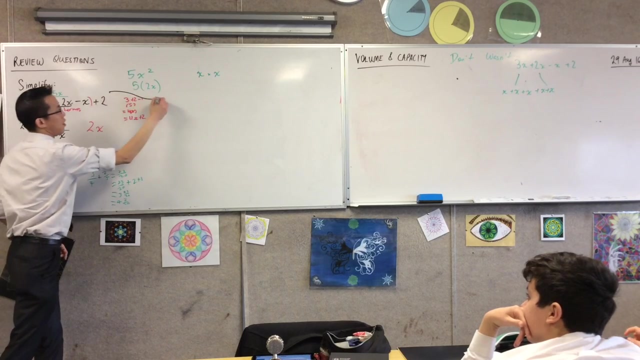 That are both hiding there and we don't write them because we just want to be quicker. yeah, So you took away one of them, which is why we get four, and then there's this two hanging over. Does that make sense? Can I also encourage you? just have a look. See the way this has been set out here. I understand what's going on. It's kind of like what's happening in your brain, but can I encourage you to write it a little bit differently? right Over on the right hand side here, I asked you to rewrite the question if you haven't already. Here's how I'm going to set it out. 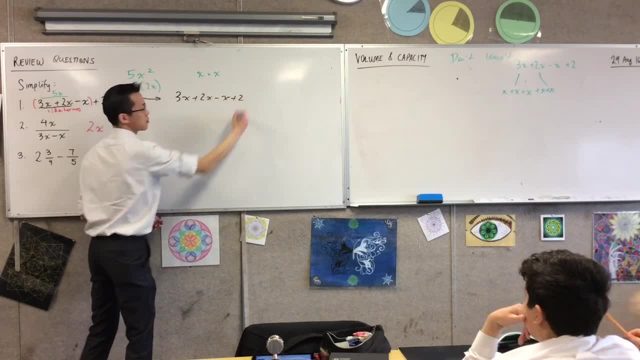 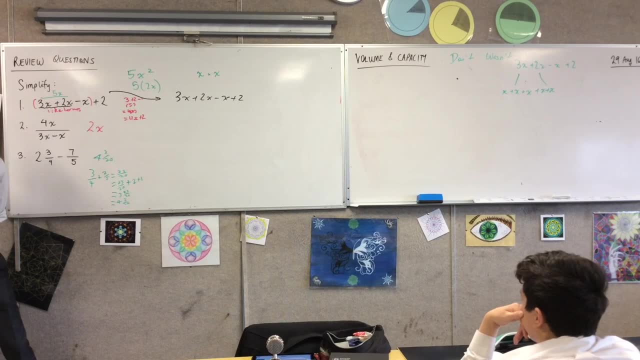 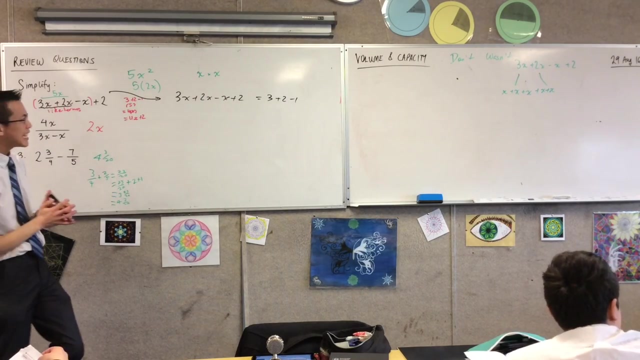 I've got 3x plus 2x, takeaway x plus 2, okay, Now is this equal to 3 plus 2 minus 1?? Is that the same as this? Yes, No, Yeah, so there are two problems with this, right, There are two problems. Number one: see this plus 2, this guy over here. What happened to him? 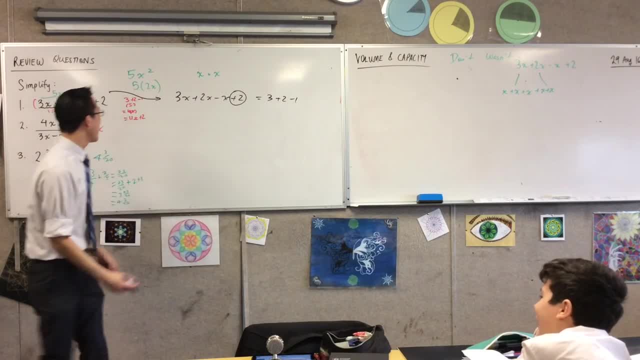 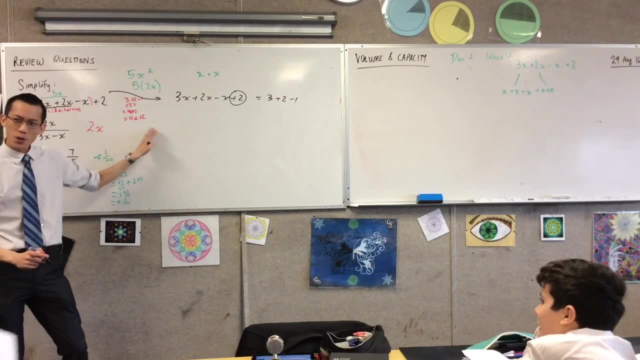 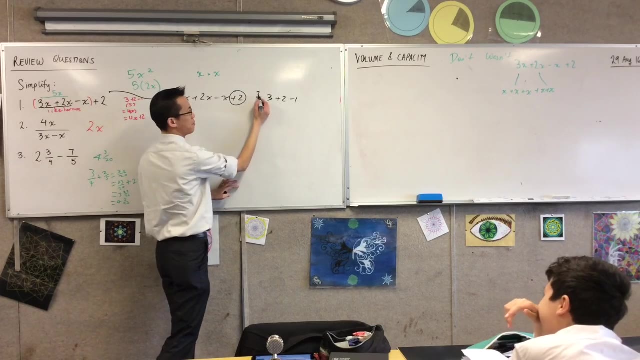 He just disappeared right, And then you notice he made a sneaky reappearance. He did come back right, But if he goes away and comes back, then this isn't really true, is it Right? It's like kind of equals, right, But not really. 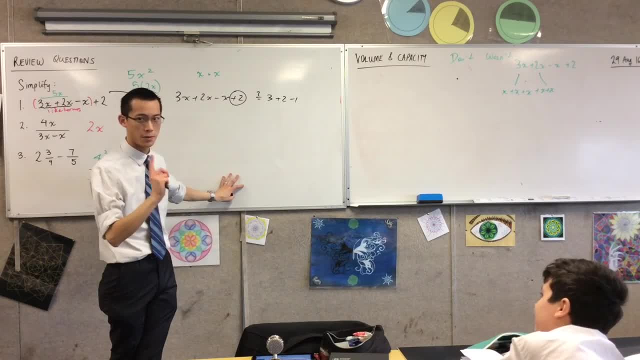 Okay, there's the first problem. What was the other problem? That's the first one. What's the other thing? that's disappeared. The x's have all just vanished. Yeah, the x's have all just vanished. Now I get why: because we're thinking about the numbers. 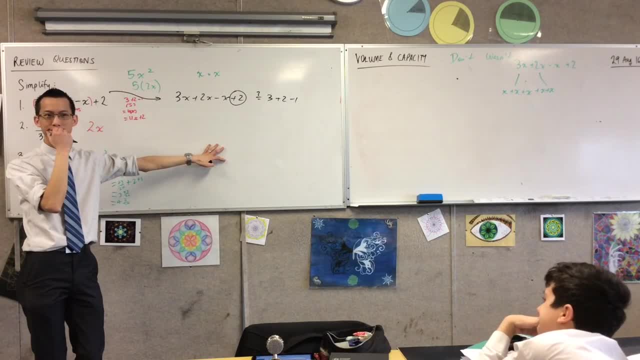 Yeah, the x's have all just vanished. Now I get why, because we're thinking about the numbers, But do we know what it is? This is a major thing in the CATII as well. This is a major thing in the CATII as well. 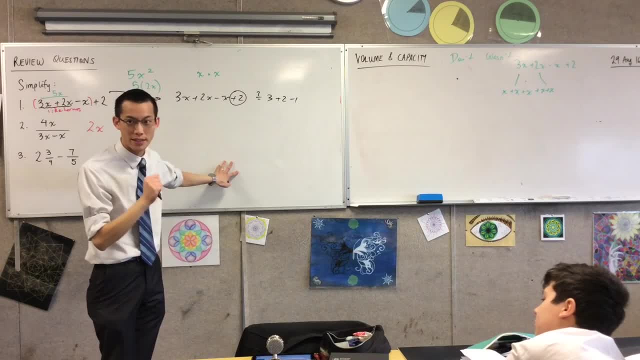 It's not ready to give back to you today, but I want to point it out right now. It's not ready to give back to you today, but I want to point it out right now. When was it Give me? Two weeks ago, last Wednesday. 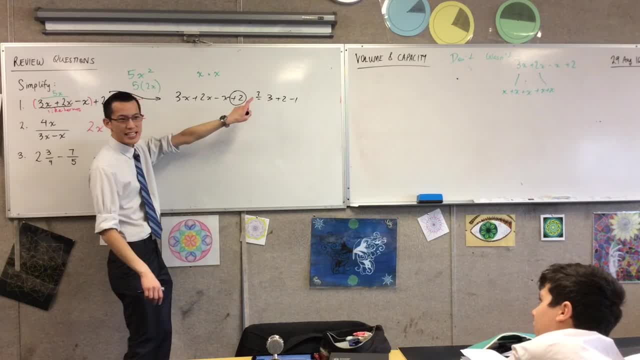 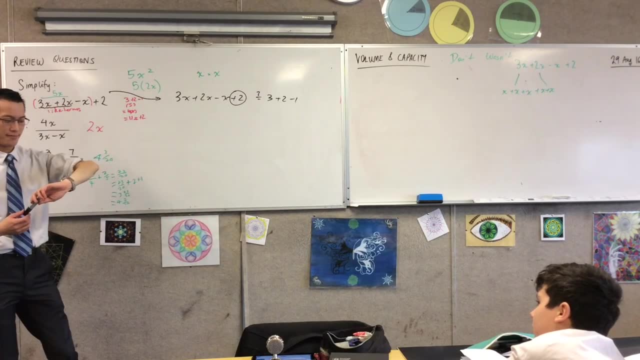 If I want to say these things are really equal. If I want to say these things are really equal- Oh interesting, I'm really literally okay to do this at lunch time, Like I don't mean that as a punishment thing. 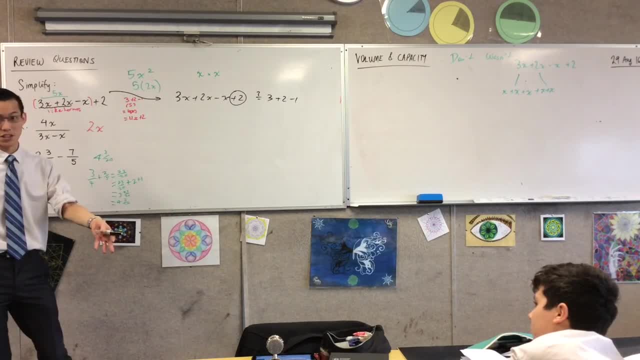 I just mean that as a run-out-of-time thing, I'm happy to have the conversation with you. I'm not doing anything in much time, But I expect you probably are, And I'd really love you to understand this. come out of here with a good understanding of this. 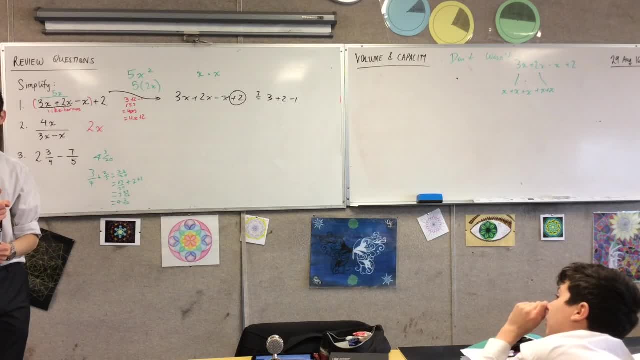 a confident understanding of this that it takes some time and attention. Do you think that's reasonable, Year 7?? Let me just double-check that. Do you think that's reasonable, Year 7?? Yes, Okay, That's better. 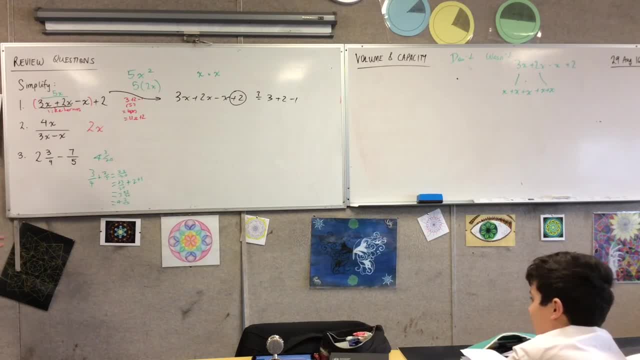 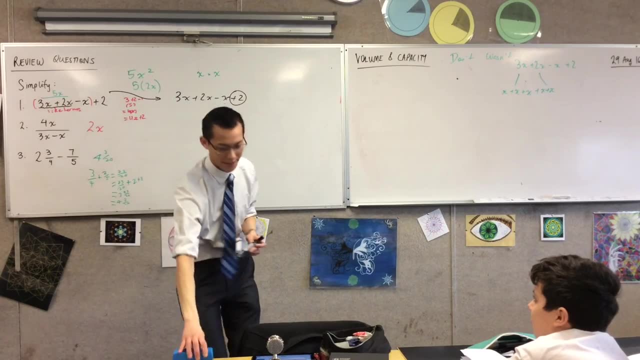 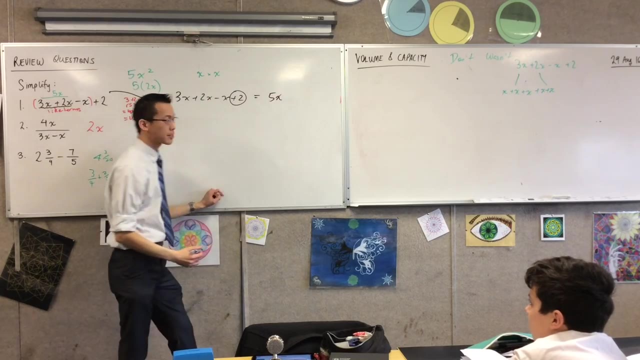 Let me see you put your money where your mouth is. If you really want to say that's equals, write this with me please, On the right-hand side of this equals sign. Let's just do this one step at a time. We've just convinced ourselves that 3x plus 2x is truly 5x. 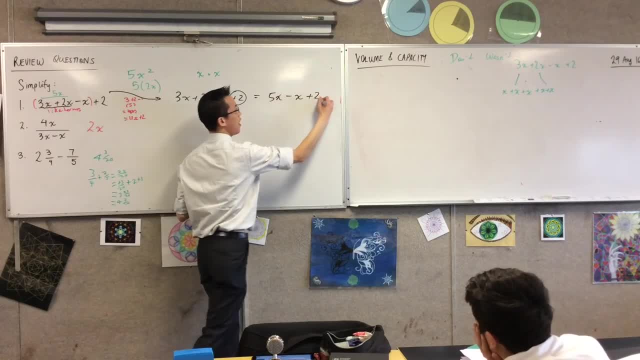 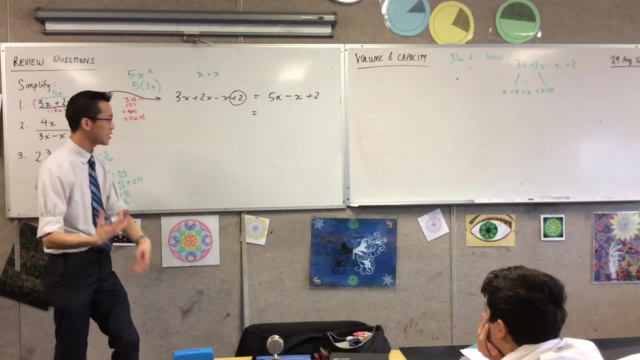 But then there are these other things here, So I need to include them, Otherwise it's not really equal right. That's what that sign means, But I want to keep working on it, I want to keep doing more things with it. 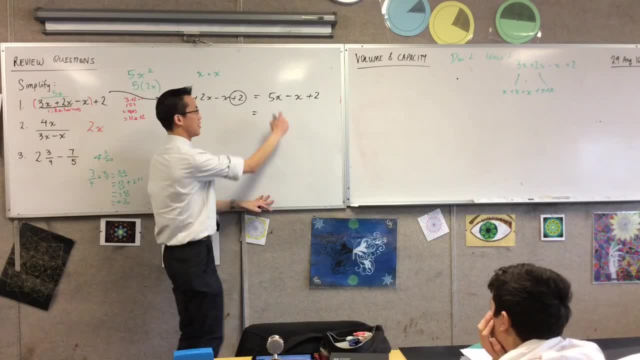 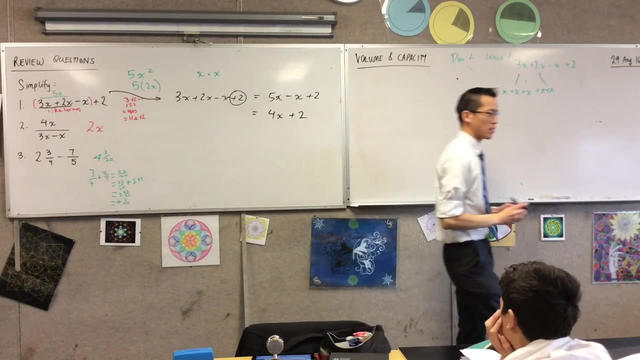 So I'm going to write something else that's simpler but still equal. So I'll write this: I'll deal with these guys like that And the plus 2 just hangs out on the end. Why don't I do anything with the plus 2?? 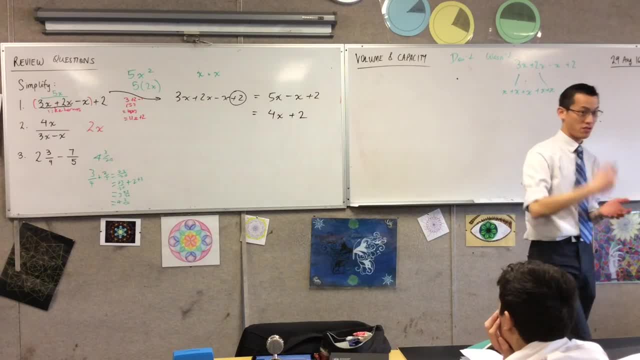 Why doesn't it get added to the 4?? What do you reckon, Jordan? Because it's not 2x, it's just 2.. Yeah, very good. Jordan very helpfully said: yeah, these are like terms. These guys are similar, right. 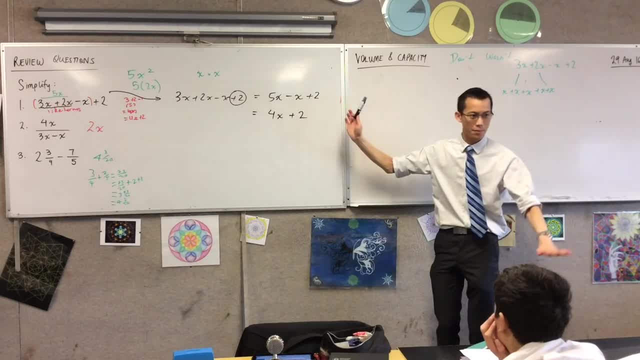 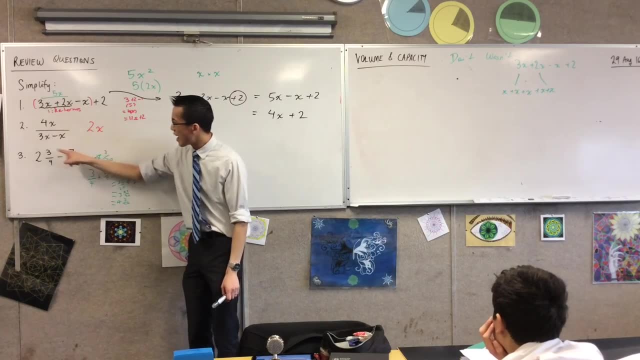 They're x's, They mix together, But this guy over here is separate. All right, We'll do the rest of the questions a little bit quicker, since we dwell on that one a little bit. This, in fact, I think you'll find, is actually: 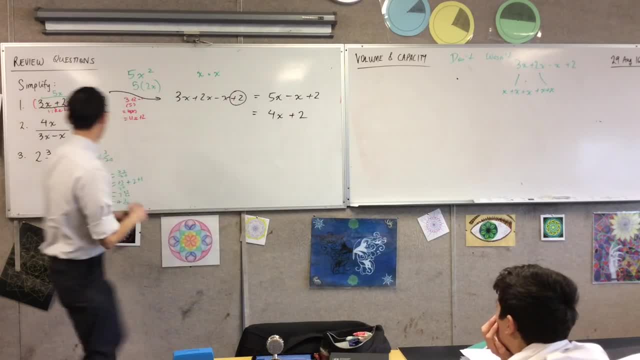 This, in fact, I think you'll find is actually 2.. Not 2x. Let me try and convince you Again. I'm going to do it with working out. So on the top it's 4x. 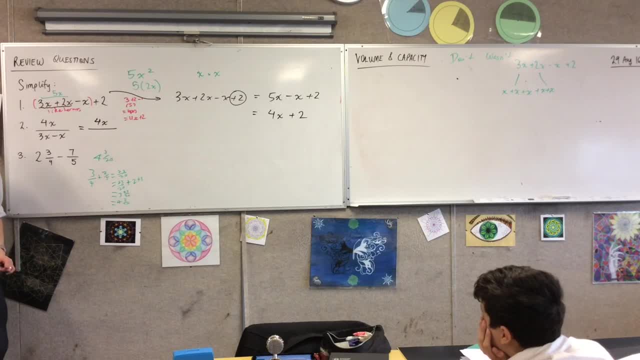 What does this sign mean? again, What does that mean? It's division, right? So I'm dividing by whatever. this is 3x. take away: x is 2x. Now you can see here, right, If I gave you just a fraction 4 over 2, just by itself, you'd all tell me that it's 2, right. 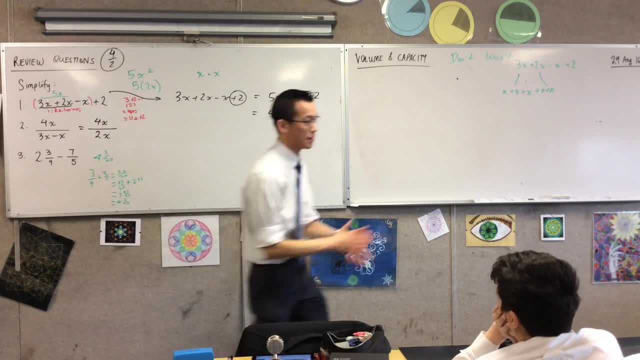 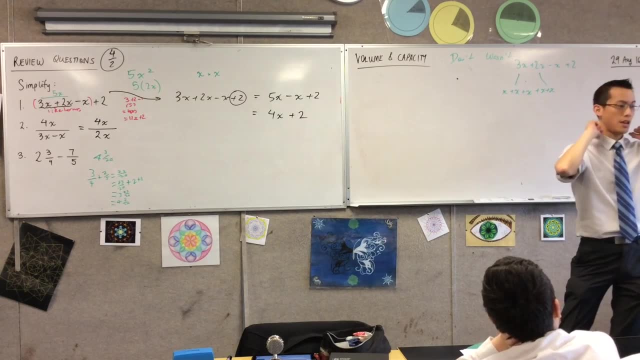 Now remember: x can be anything. x can be anything. Okay, Let's suppose x were 10.. Suppose x was 10.. If x were 10, the numerator is going to be 40. If x is 10, the denominator is going to be 20.. 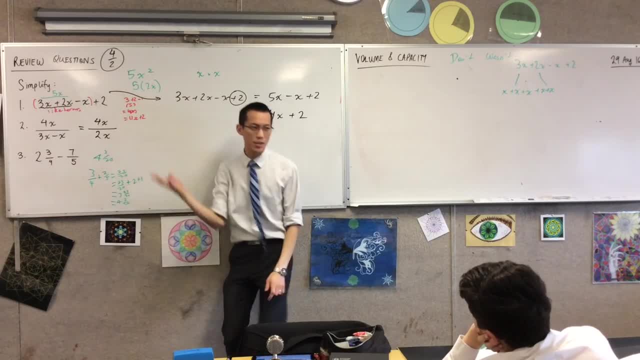 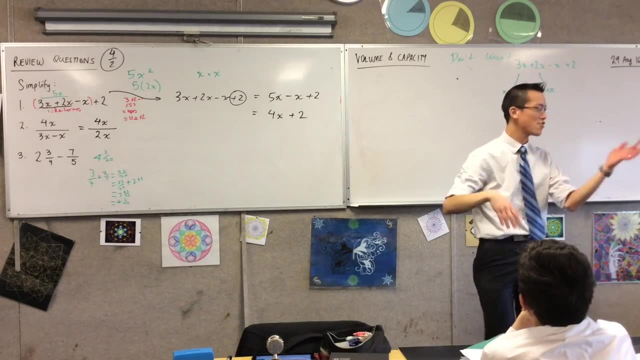 It's still going to be 2, isn't it Right? What if x were 100?? 400 on 200.. What if x were a million? Okay, You get the idea right. It's always: whatever x is, it's always going to be 2.. 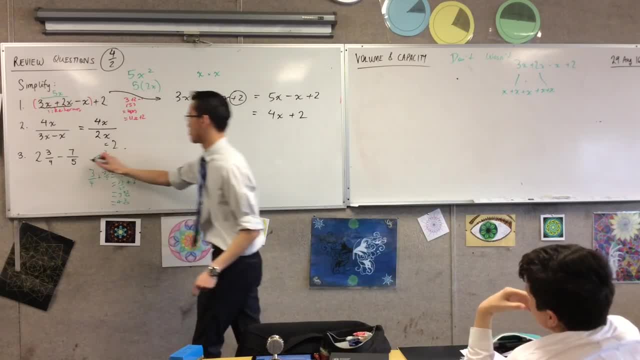 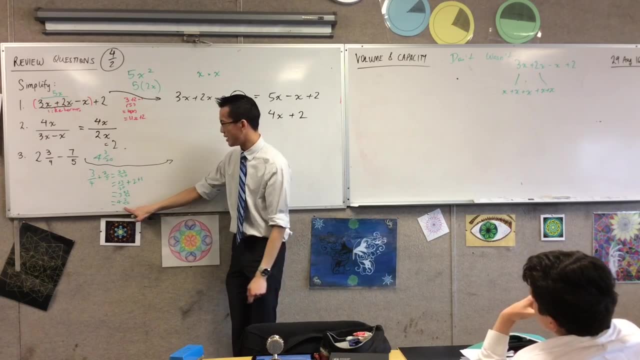 Okay, Now this line is going to be 2.. So this last one. I think something has gone a little funny, partly because I feel like our answer is bigger than what we started with. but I'm subtracting, So let me try and do this. 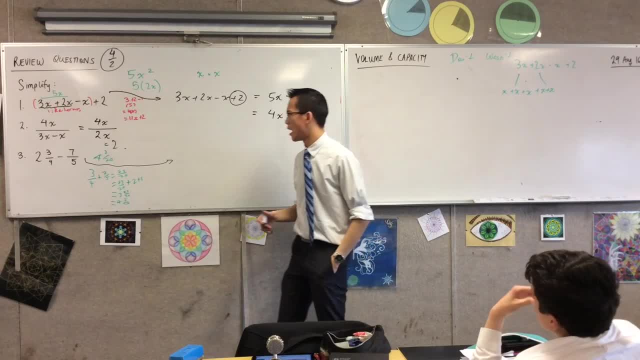 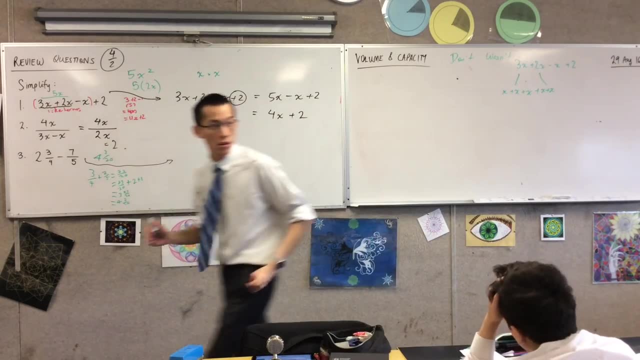 I don't know what the answer is yet. by the way, Let's try and do this together. What do you think the first problem is with these guys? I can think of at least two. Yeah, Christian, One of them is mixed and one of them is in the proper order. 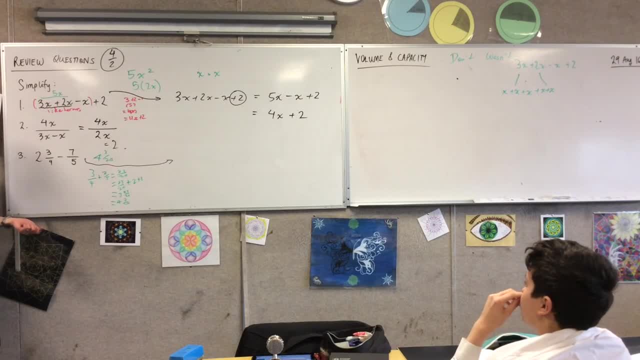 Yeah, okay, So that's a bit gross, right. So let's get them both. How about we get them both? Actually, which would you prefer? We could do both. We could do either. I mean, Do you want both mixed numerals or both improper fractions? 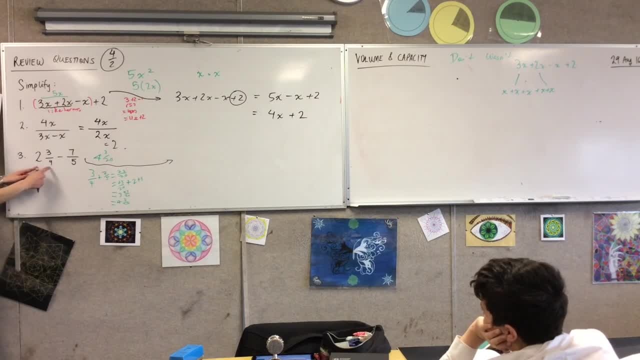 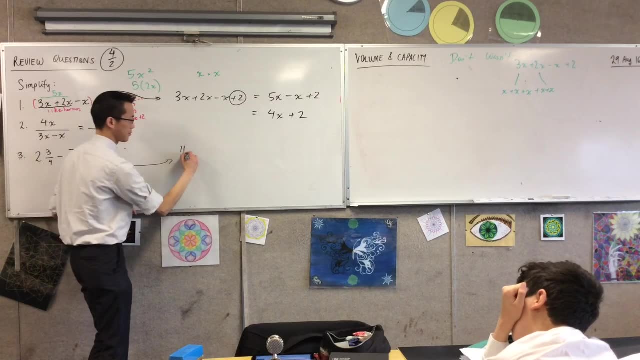 Which would you prefer? Improper, Improper, Alright, let's do it. So what is this as an improper fraction, 4 times 2?, 8. Plus the 3?, 11. 11 and 4..